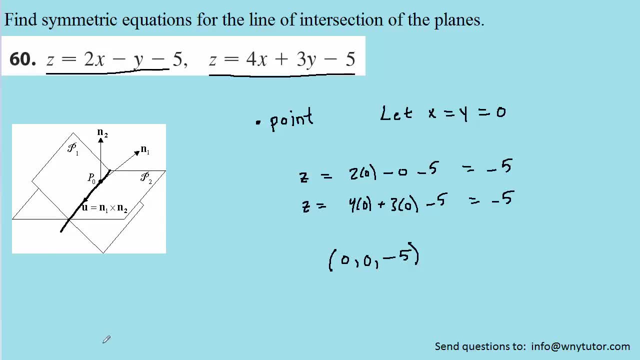 line, or is at least parallel to our line, And so to find that vector that's parallel to our line, it's going to be helpful to take advantage of the following fact, And you might want to pause the video and read this statement a couple of times: The statement mentions that the cross product of 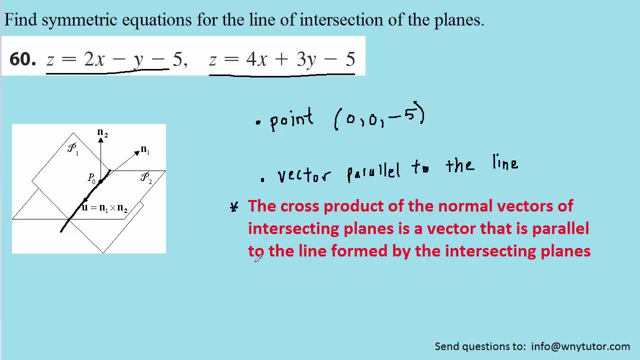 the normal vectors of intersecting planes is a third vector that is parallel to the line formed by the intersecting planes. Now the normal vectors are shown in the diagram. This normal vector, marked n1, is perpendicular to the plane that's marked p1.. And then the normal vector n2 is: 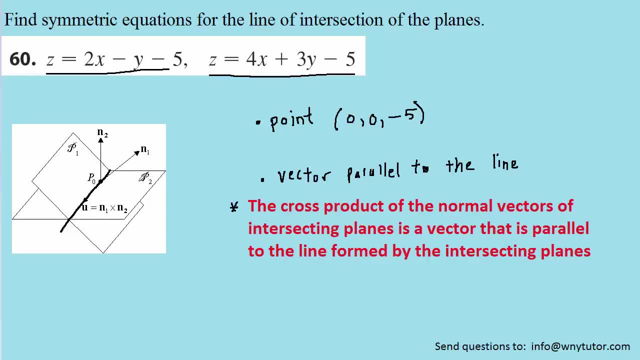 perpendicular to the plane that's marked p2.. And when we multiply them using the cross product, we're going to get a third vector that will automatically be perpendicular to both n1 and n2.. And by being perpendicular to those two normal vectors, that third vector will 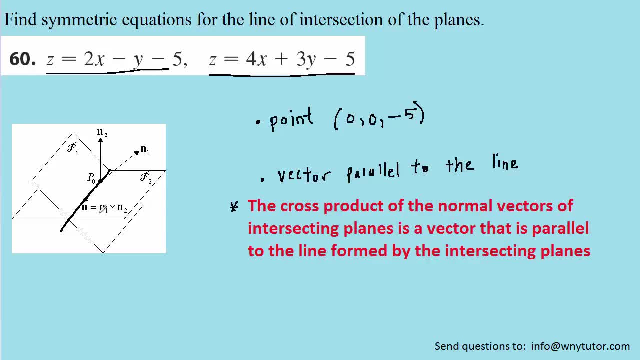 automatically run parallel to our line. So, in essence, to find that vector that's parallel to our line, we're going to need to find the cross product of intersecting planes, And so to find that vector that's parallel to our line, we have to take the cross product of these two. 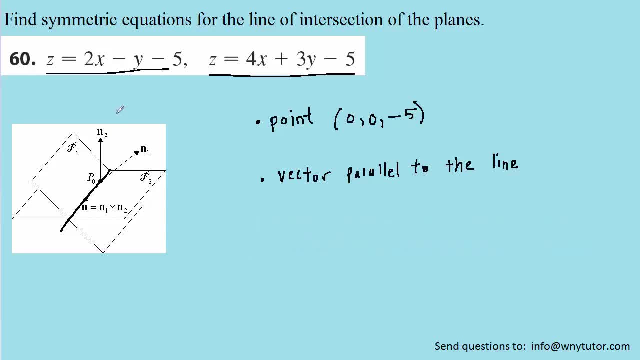 normal vectors, And so our next step is to find the normal vectors n1 and n2.. What we need to do to find those normal vectors is get our plane equations equal to zero. So if we subtract z from both sides of this equation and organize the terms in order x, y, z, we could see that 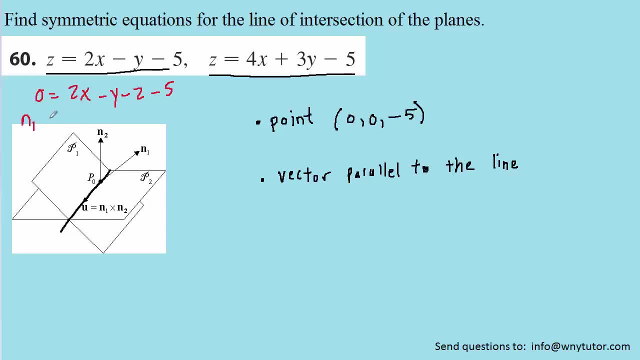 the normal vector for this plane- we'll call it n1, would simply be the coefficients of x, y, z. So we would have two, negative one and negative one. In a similar manner, if we subtract z from both sides of this equation and organize the terms, we can see that the normal vector that 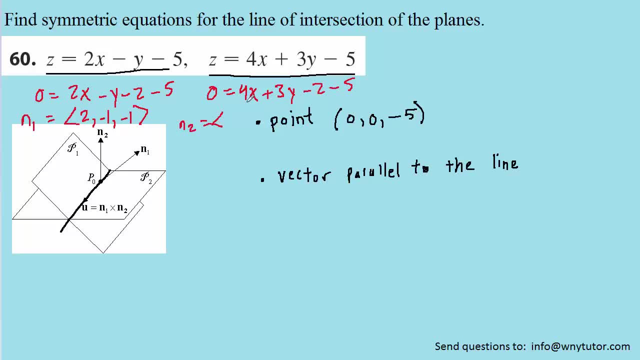 we can call n2, by looking at the coefficients will be four, three and negative one. This is a negative z right here, and the coefficient is negative one, So we can write that as n2.. Now that we have those two normal vectors, we can write the'. 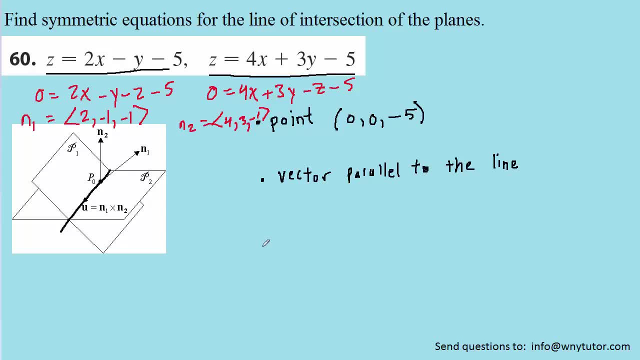 vectors. we can go ahead and set up the cross product, And to set that up we simply put in the normal vectors n1 and n2.. n1 will run in the first row, and so we can put in the 2, the negative 1, and the negative 1, and then n2 will run. 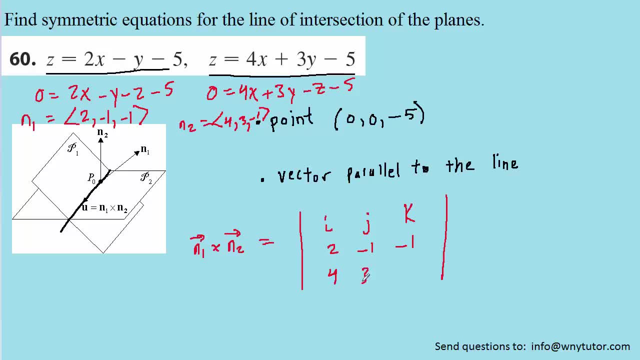 along the second row, which will be 4,, 3, and negative 1.. Now, when doing a cross product, we end up with both an i component, a j component and then a k component. We do have to remember that between the i and j component, there will 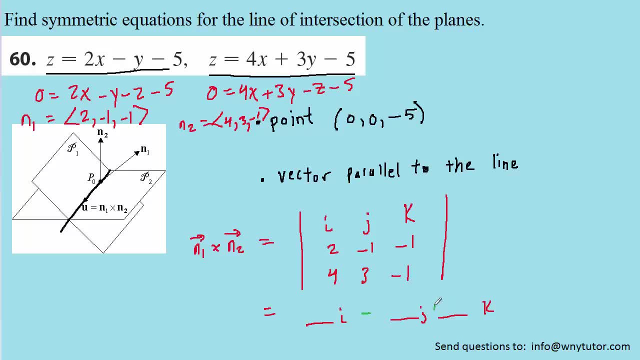 be a subtraction sign, but between the j and the k component there will be an addition sign, And then we can actually perform the cross product. Now for the i component. what we're going to do is actually cover up the column that is marked i. 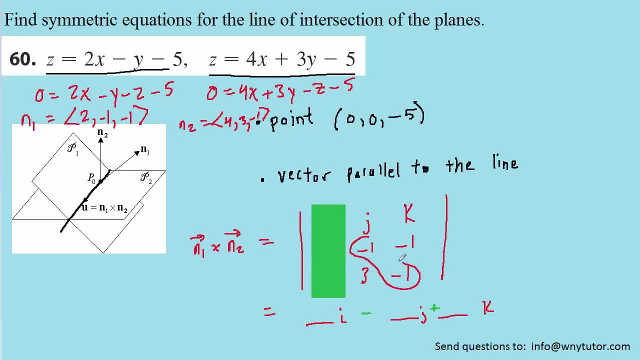 We then essentially do what I like to think of as cross multiplication. So we do negative 1 times negative 1, which of course is 1, and then we subtract the cross multiplication going the other way. So 3 times negative 1 is negative 3, and 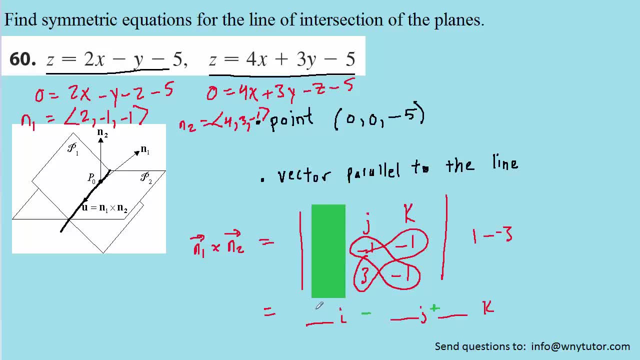 1 minus negative 3 will be positive 4.. So we're going to put a positive 4 for the i component right here, And then for the j component, we can cover up the column that contains j. so this column right here, And then, once again, we'll do some. 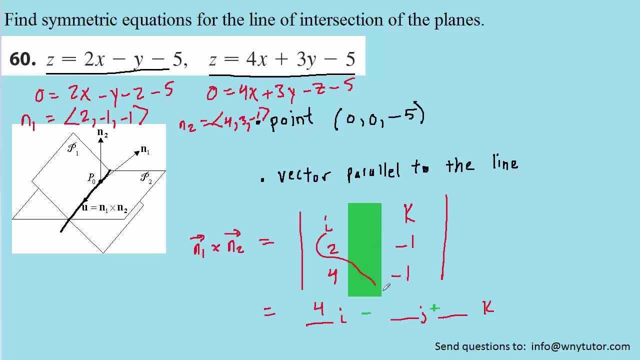 cross multiplication. So 2 multiplied by negative 1, of course, is negative 2, and then we subtract 4 multiplied by negative 1, which is negative 4.. And then negative 2 minus negative 4 will make positive 2.. So we'll make positive 2 here for the j component, And then of 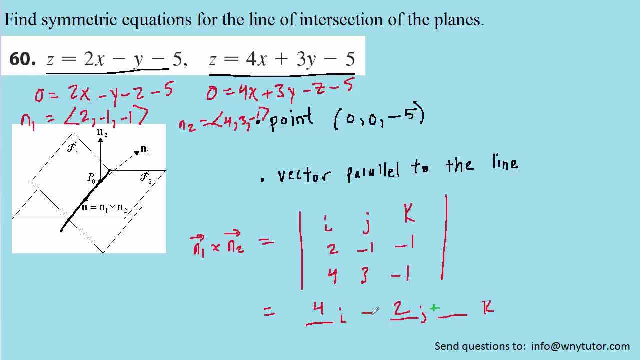 course, because of that negative sign, it actually does become a negative 2.. Finally, we will cover up the column that has k. We will then multiply 2 times 3,, which gives us 6, and then subtract 4 times negative 1,, which is negative 4, and 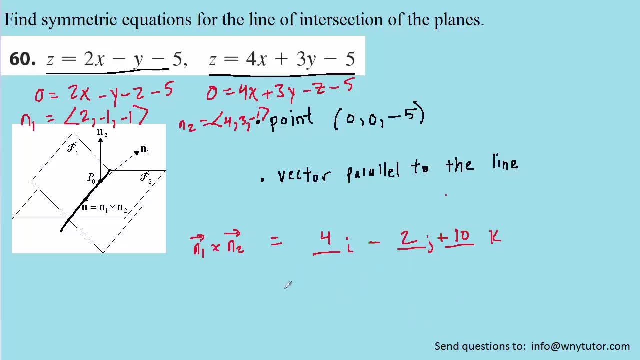 so we end up with 10.. And of course, this vector can be written in component form as 4,, negative 2, and then 10.. It's also customary to factor out a greatest common factor, if there exists one in this component form. Now, in this case, we could factor out a, 2, and 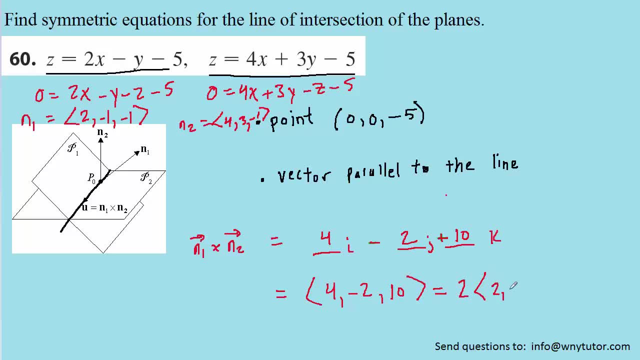 that would leave us with a component form of 2, negative 1, and 5.. And it's alright to do that, because this vector will actually run parallel to this vector, since they are a multiple of each other, And so we can use this. 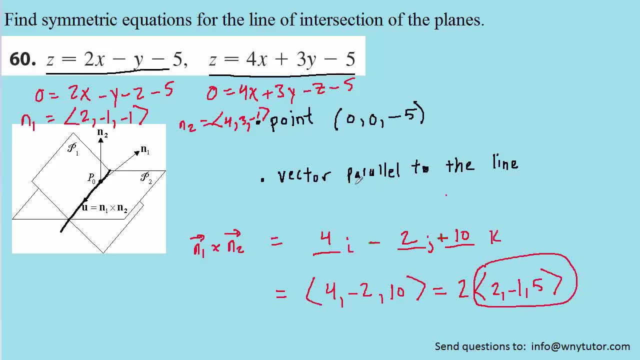 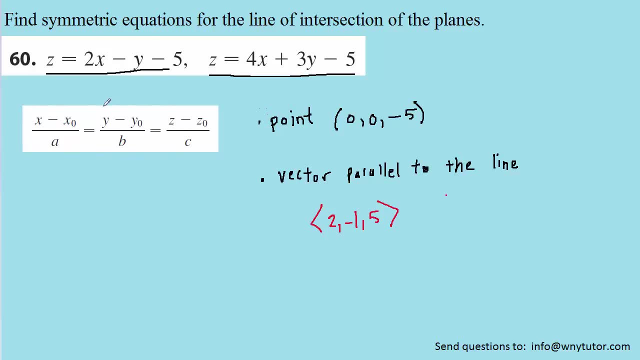 vector as the vector that is running parallel to our line, And then we can take this information and insert it into the symmetric equations for this line of intersection. Now, in the symmetric equations, we just need to note that the point is going to be x naught, y naught and z naught, And you can see those.